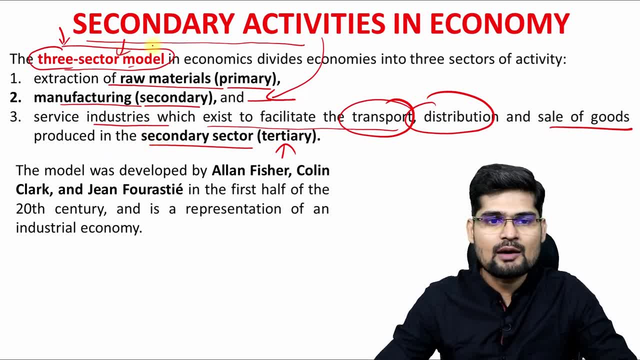 sector model is important to understand And out of which we are learning the secondary part, because in the previous lessons we have already learned about the primary activity. So this model was developed by Alan Fisher, Colin Clark and John Foresti in the first half. 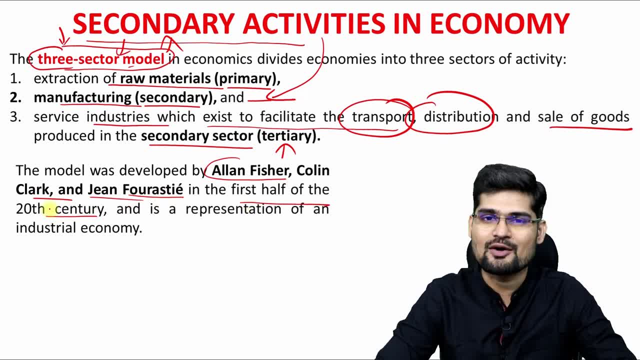 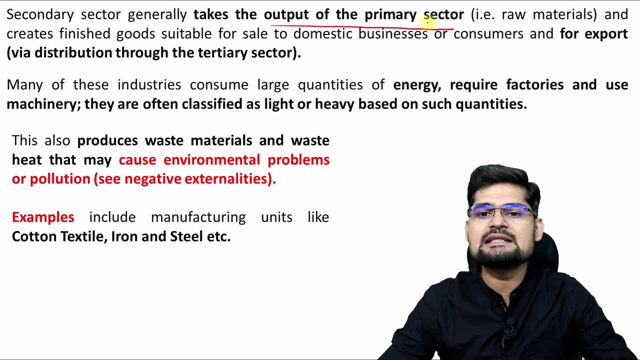 of 20th century as a representation of industrial economy. That's important to take from here. Now, what is secondary sector? It basically takes the output of the primary sector. It means what the primary sector contributes as a raw material source for the secondary. and secondary sector does what The processing part. So what does the secondary sector do? It basically takes the output of the primary sector. It means what the primary sector contributes as a raw material source for the secondary and secondary sector does what The processing. 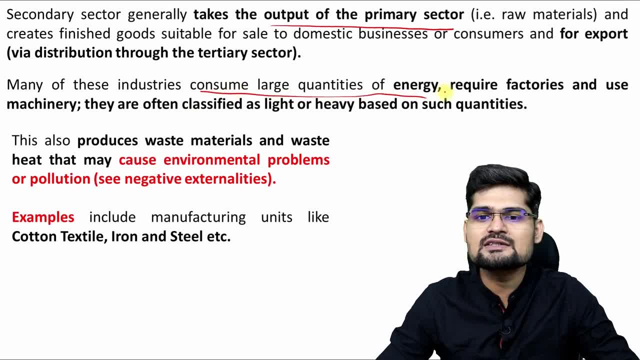 part. That's how it works. So many of these countries consume large quantities of energy, require factories, use machineries to convert the primary resources, the raw materials, in order to make it fit for the market, for the processing. So that's important. So the secondary, 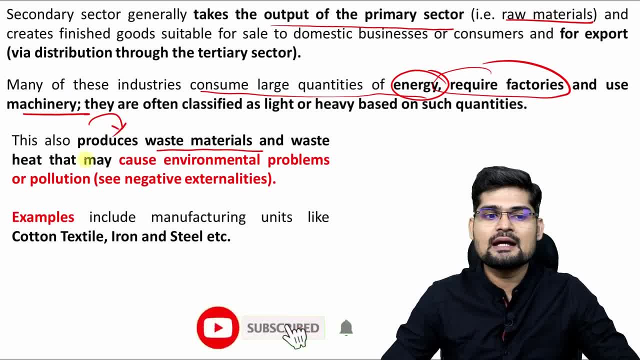 sector what it produces- Waste materials as well- And remember- this is one important point here in terms of environment as well- that this is the chunk of secondary sector that produces too much of environmental waste and causes environmental problems as well. So the flip side is it gives us resources, manufactures resources for us, but at the 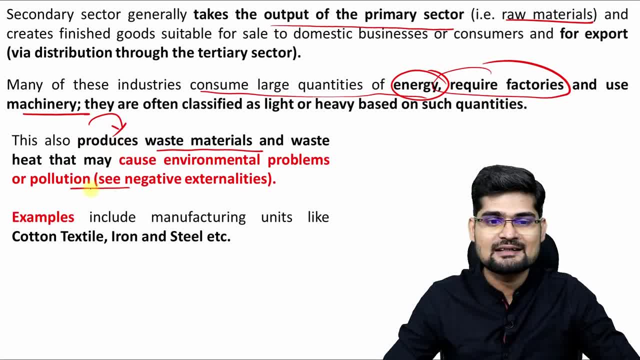 same time, there is environmental concern because of this side, right? So this is important. So example: you can see cotton, textile, iron and steel and several other industries, right? So what happens? Secondary sector is dependent completely on the primary sector for its raw 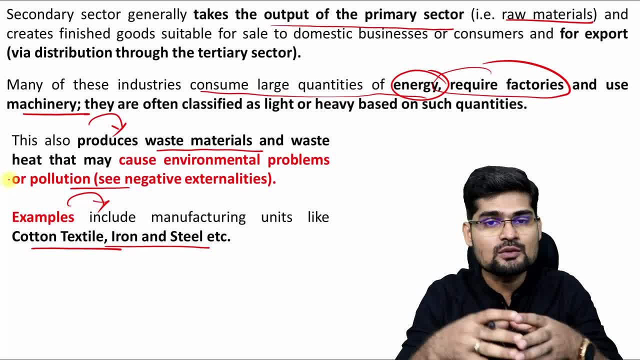 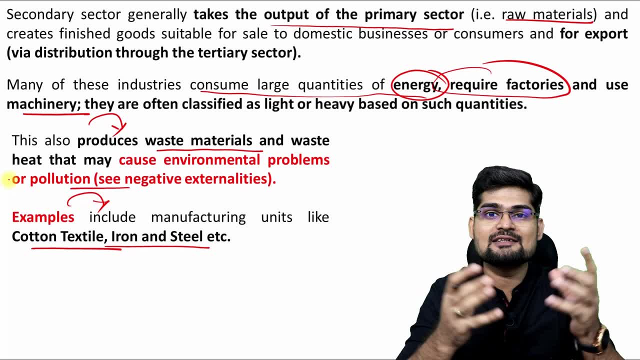 material supply. But secondary sector has life of its own because it's manufactured, It's a manufacturing unit, It has factory setup and also it requires capital, It requires finances, It required other supports like transportation and other logistics support. right, That's how secondary sector operates. So secondary is not in itself independent. 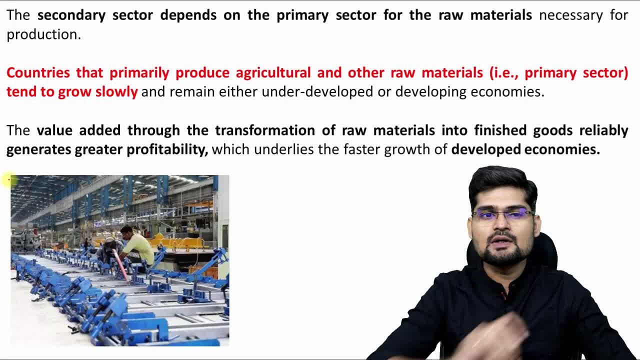 It means it is dependent on the others. That's how it works. So secondary sector is dependent sector on primary sector for the raw material, as we have discussed, and countries that primarily produce agricultural and other raw materials, which is basically primary sector. So secondary- 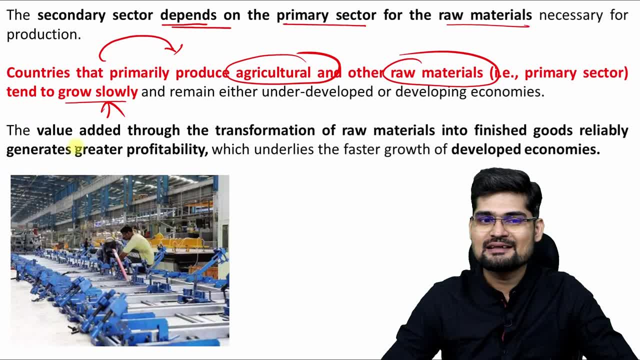 sector tend to grow very slow. that we have seen through economy right And remain under developed. that we said. that we also know by the name of developing economies. But remember the countries which produce the goods out of these raw materials that is dependent upon. 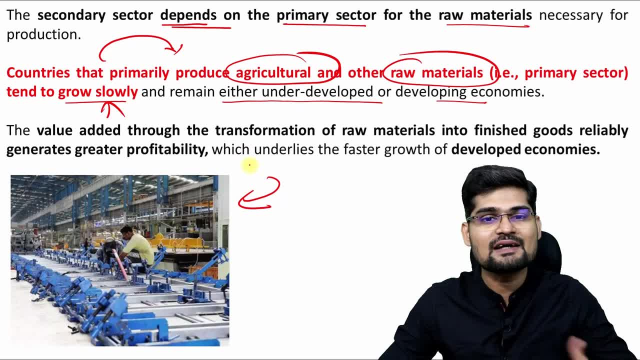 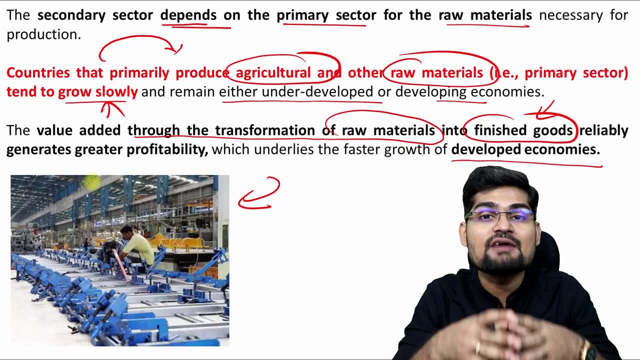 secondary sector or domination of secondary sector or manufacturing sector. these countries become developed very fast, right. So value added through transformation of raw materials into the finished goods which comes to our home. Finished goods have better advantage and also value. that we say right. So that's why. 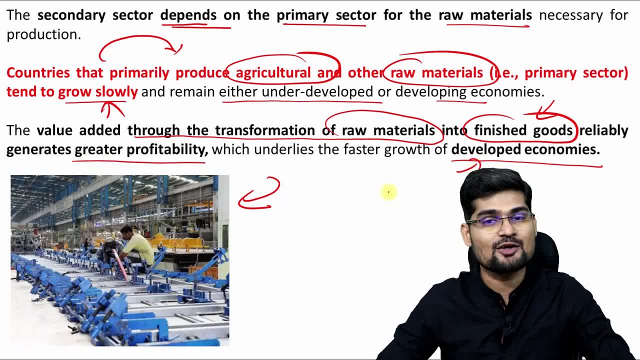 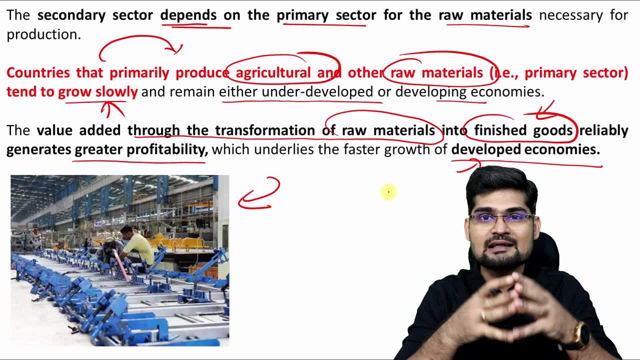 it is greater in profits, which leads to faster economic growth. That's why secondary sector is very important In India right now, we're trying to emphasize on homegrown goods, right Home produced material from our own factories, made in India. That's why we have programs. 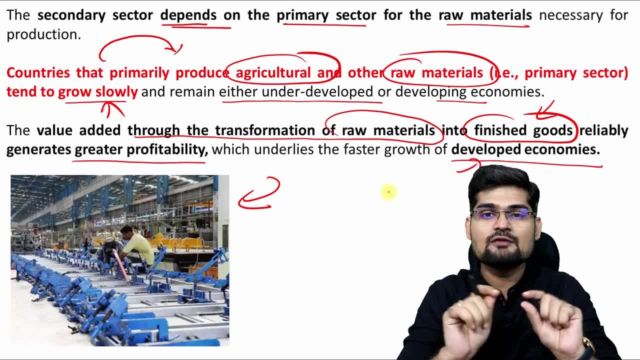 like Skill India, Startup India and several other programs where we want to make in India concept to come alive and also lead in various aspects. right. So that's the whole idea we want to develop as manufacturing hub. right, Because it would lead to the path of development. 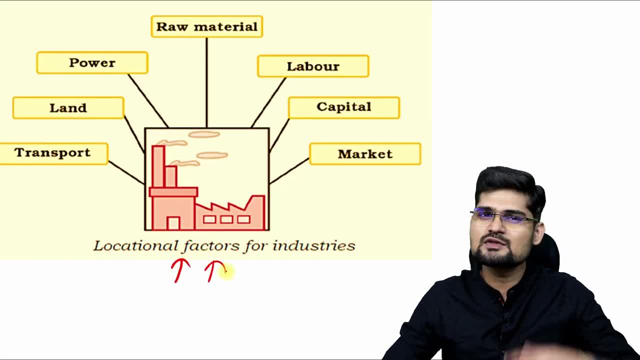 So the whole idea is, if you observe these locational factors for industries which we have talked about in the previous sessions, also for industries for manufacturing, these seven things are very important. Top is the raw material which is coming from where. 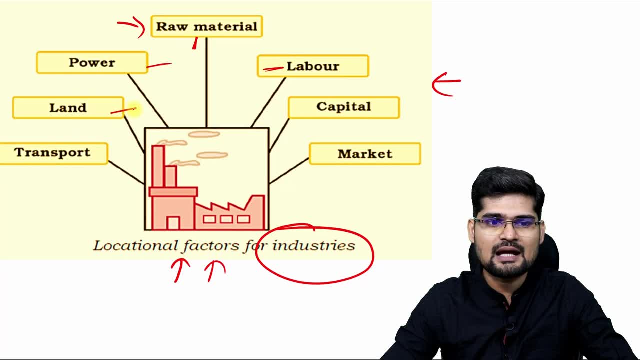 From the primary sector of economy. Then you have power, labor, capital, land, market, transport. All these things needs to come together to actually make the secondary sector sector, or the industrial sector, work and locate in a particular place. right, so classification of 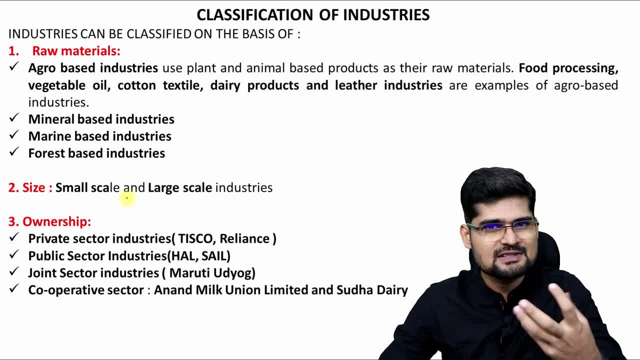 industries, if you see, because we are talking about secondary sector and industries lead in them. so classification is based on various types. one is on raw material, one is on size and one is on ownership. three things, three words. you have to remember: raw material, size and ownership, right, 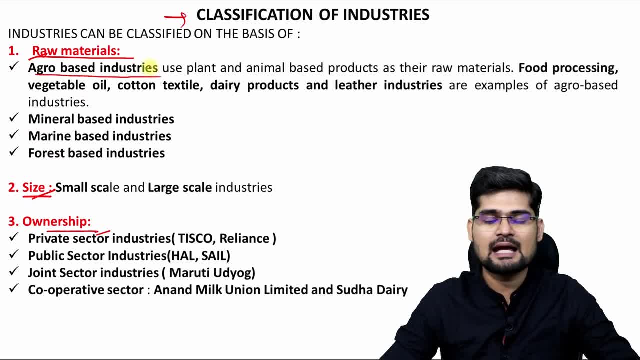 so raw material is agro based industries, for example, it is agricultural produced raw material which is taken for the processing. so we have vegetable oil, cotton, textile, dairy product, leather industries, food processing industries which take raw materials and process them into finished goods. then we have mineral based industries. we take minerals and produce different objects from it. 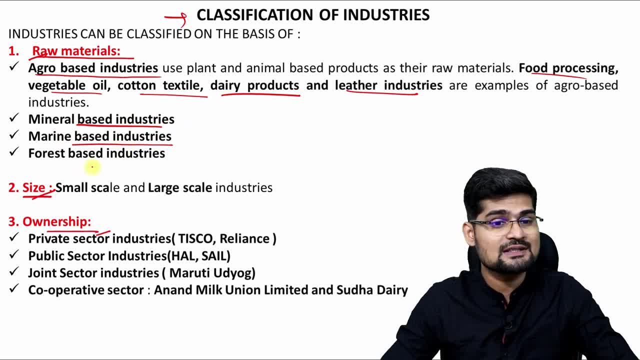 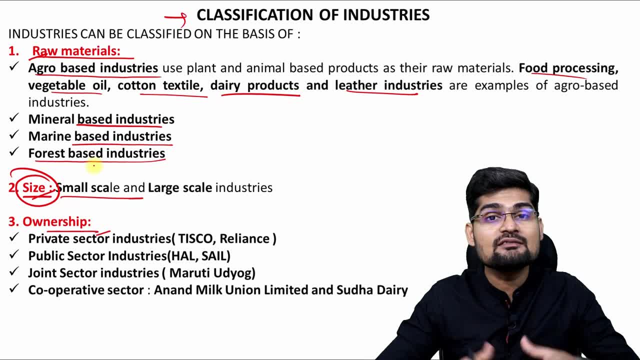 does it require and how much is its output in output, in productivity? the size also is there right. so it's kind of a scale concept. so small scale or large scale industry? right then comes the ownership. the third one, that is, who is owning it? is it privately owned sector, for example tisco? 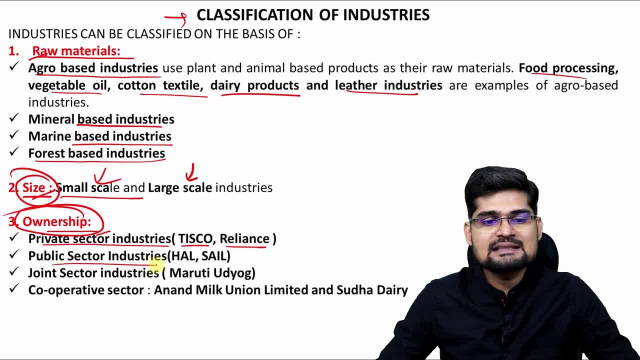 reliance right, which is in private hands, then public sector enterprises like hal sale right, so these are public sector units. then you have joint sector units like maruti uddio right, where you have combination of public and private, and then you have cooperative sector as well. for 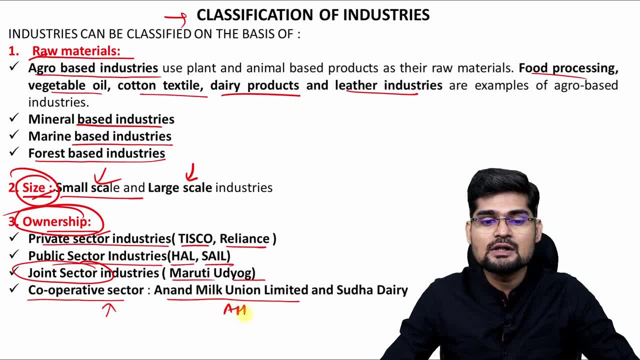 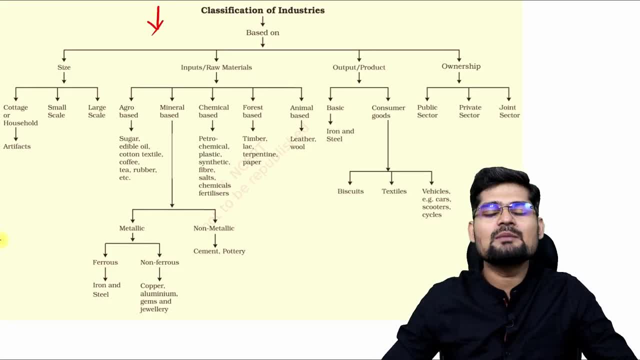 example, remember the anand milk union, limited amul that we already know, operation flood and also sudaha diary, now looking into classification of industries through a flow diagram. you can make this flow diagram and learn from this as well, if you don't want into the text. so it is based on. 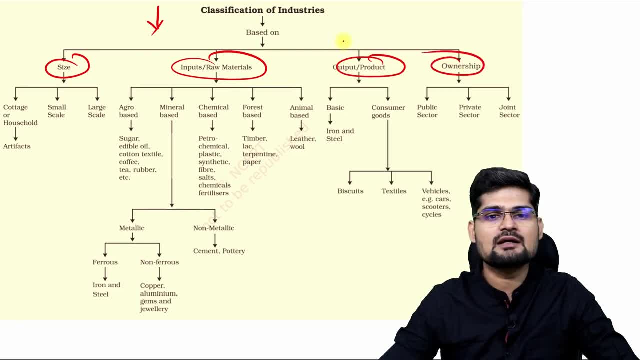 size, raw materials, output and ownership. there are these four classes here, right? so cottage or household, small scale, large scale, artifacts, which is part of this size classification. then in input that is based on raw material, you have agro based, mineral based, chemical based, forest based, animal based. so five types. if you see, examples are given here. you can. 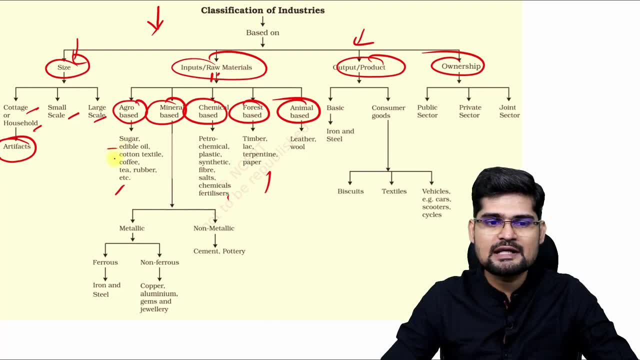 pause the video and you can note it down for yourself. sugar, edible oil, cotton, textile, coffee, tea rubber is agro right. in mineral you have metallic or non-metallic minerals. for example, non-metallic is cement and pottery industries, then in metallic you have ferrous and non-ferrous. 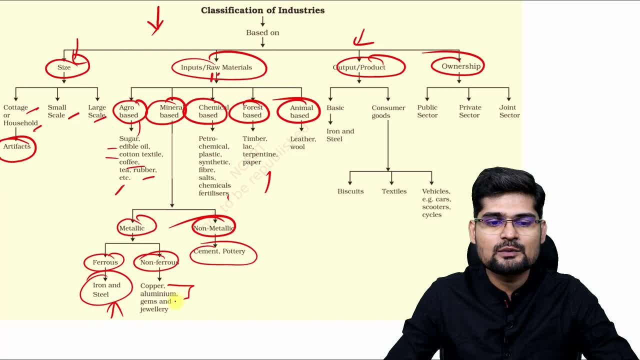 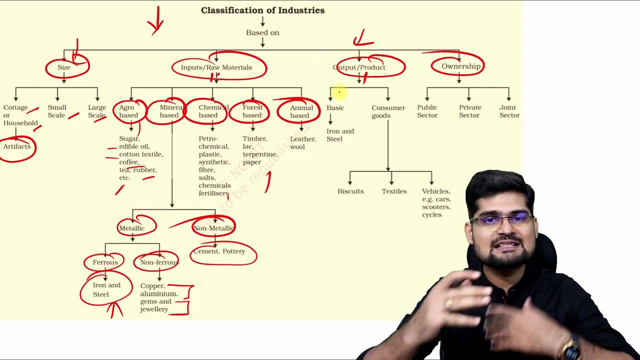 so iron and steel industry, the most famous one- and copper, aluminium gems and you know other jewelries, right, those are the non-ferrous. then, further, if you see output on the basis of output, how you classify so basic is iron and steel industry- then you have consumer goods industries. 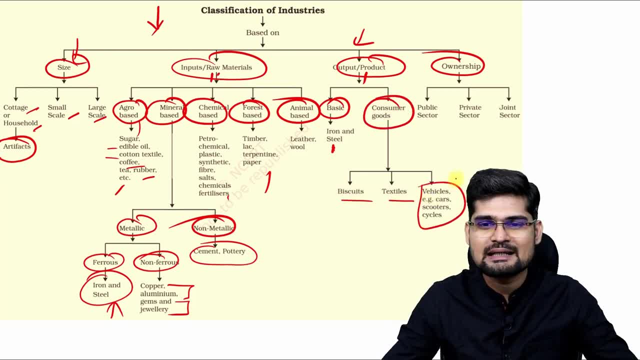 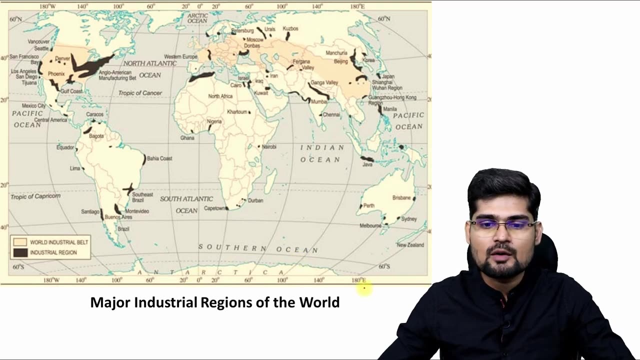 like biscuits, textiles, vehicles, for example, cars, bikes. then you have ownership based. as we know, this is here. so this one flow diagram can give you an overview as well that you can practice and learn for the classification of these industries. now comes the major industrial regions in the world. if you observe this map simply, 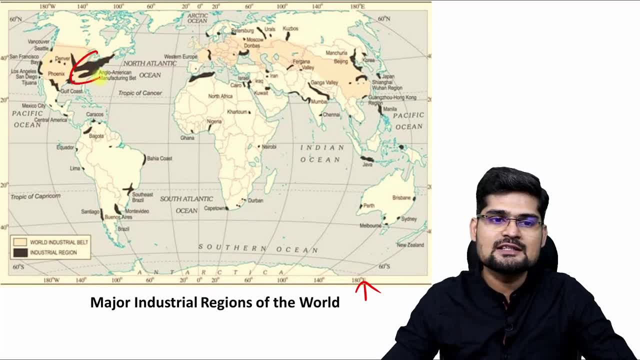 you can find out which areas in the world, if you see the east coast and here this part, the great lakes, part of us here on the west coast as well, then you have this mediterranean area somewhere in europe as well, in india as well, in other portions in southeast asia as well, right in south america. 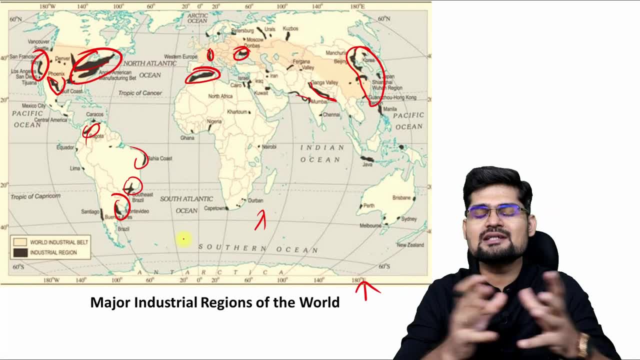 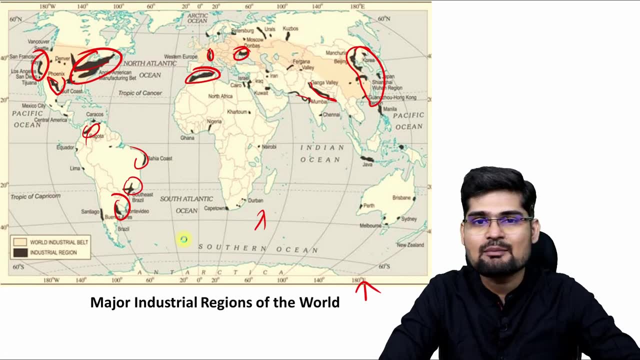 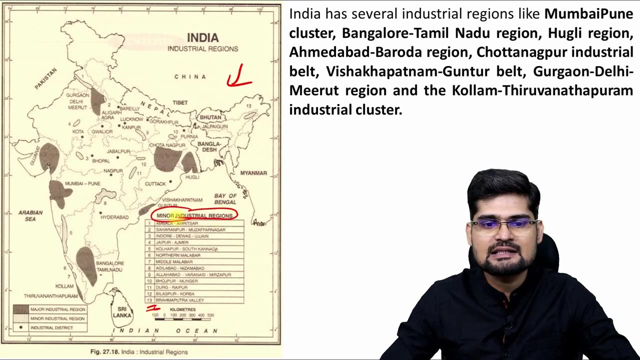 some places so largely, if you observe, this is the major industrial regions of the world on the map which you can mark for yourself and learn about it, that which are the areas which is the example. and in india, if you observe, this is very important to learn this: 13 here minor industrial regions and. 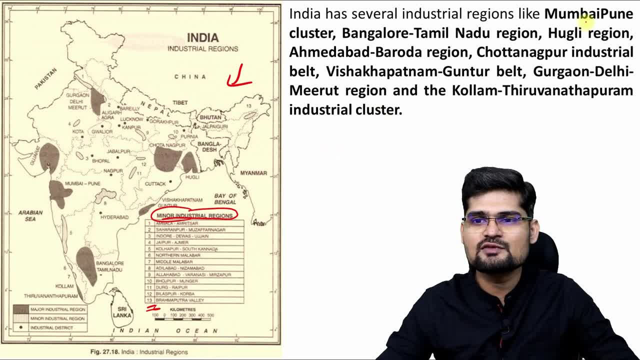 the major industrial region. so you have eight major industrial region, if you see mumbai, pune cluster, bangalore, tamil nadu region, kogli region, ahmedabad, baroda region and chotanakpur industrial region, vishakapurnam, guntur, then gurgaon, delhi merit region and column tiruvananthapuram industrial 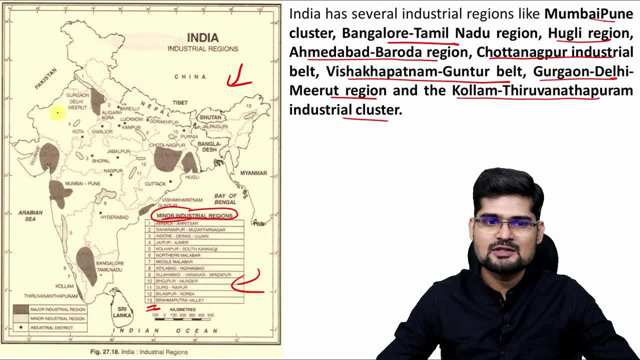 sector, right and minor, including these are 13 ones here. so if you observe at least these major chunks which you see in the dark, these major chunks, at least these major chunks which you see in the dark, you should remember, for indian example. all right, so now let's look at the case study of iron and 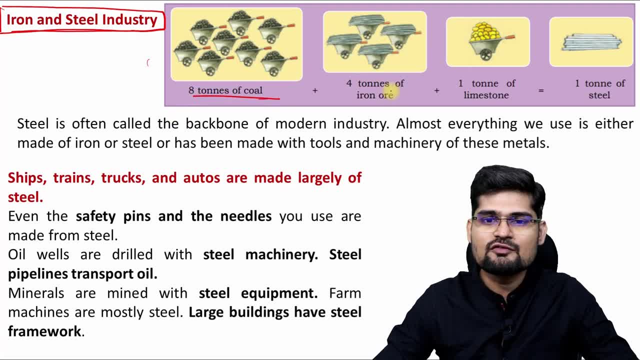 steel industry how it works. so eight tons of coal, four tons of iron ore and one ton of limestone. it means coal, iron ore and limestone combined together gives us one ton of steel. so to produce steel we need these three sources. that's how it works in secondary industries. so steel is often 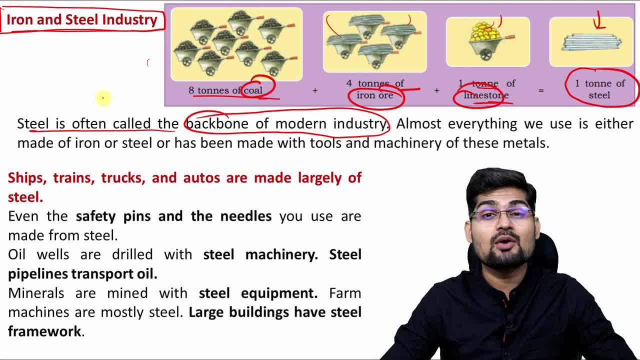 called the backbone of modern industry and modern urbanization. cities are built on steel. that we say in our everyday life, from needle to tools we use of metals, mostly of steel right. so ships, trains, trucks, autos, they are made of steel, safety pins to needles to steel, machinery, steel pipelines. 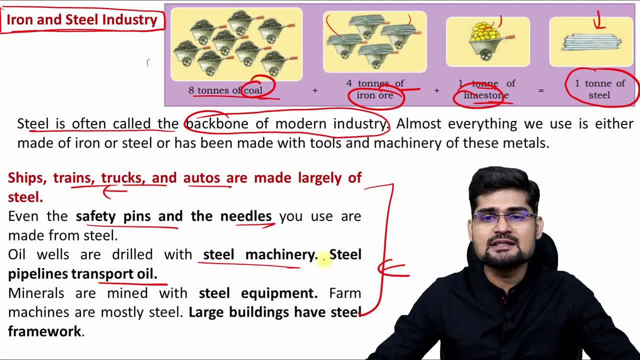 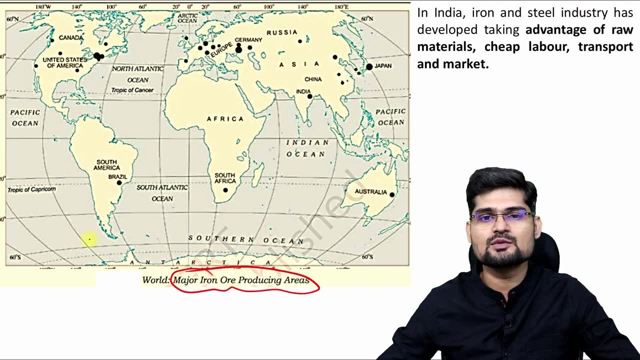 transport sector, right, everything is working on steel. so steel is the backbone of economy, that we say. that's why iron and steel industry becomes really the backbone of manufacturing industries across the world. right, so what we observe? look at this particular diagram: the major iron ore producing areas in the world. 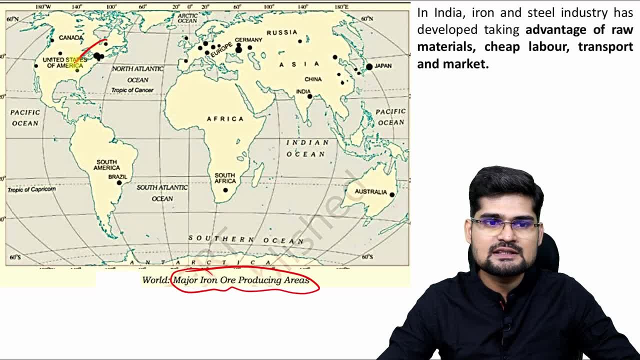 will definitely lead in steel production as well. so if you see the commercial hubs, these are the areas which are iron ore producing areas in the world, from russia to us, to india, to southeast asia, also in south africa, brazil, australia, all these places, if you observe on the map, so you find that. 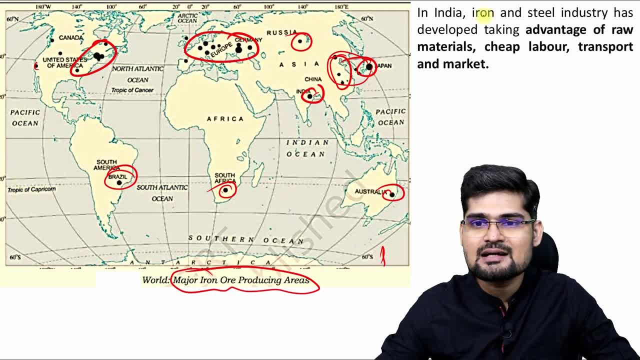 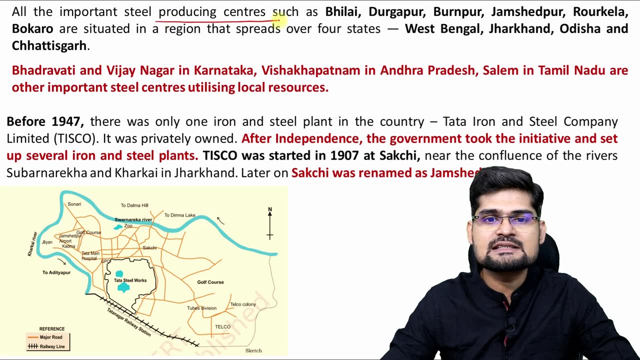 their iron ores are deposited. and in india iron and steel industry has developed taking advantage of raw materials, cheap labor and transport and market. that's very important factor. so we say these are factors of production. right now, all important iron and steel producing centers, for example, bilai, durgapur, burnpur, jamshedpur, raucula, bokaro- if you observe all of them coming. 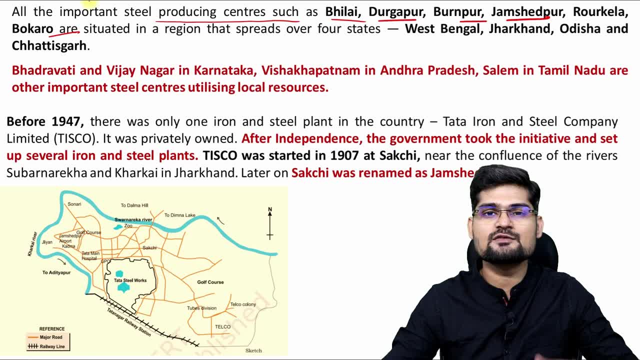 after independence: right, we had the five-year plans which were focused on the growth pole concept that if these iron and steel industries are there, then what would they do? they would strengthen our economy, our cities would bloom and gradually, development of the region will happen. right. so it is spread over four states: west bengal, new zealand, antarctic don, Atlanta, sorority, india and 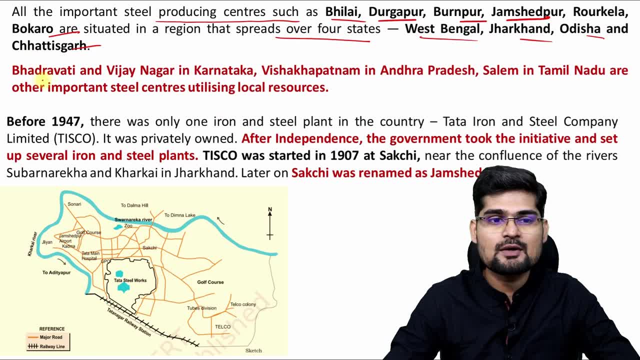 haiti, bandhmanaliaffer, damshad and kayan env. siri ghar, Gillip bastard, boelish, indian and all jharkhand, odisha and chhattisgarh, and remember bhadravati and vijaynagar in karnataka. 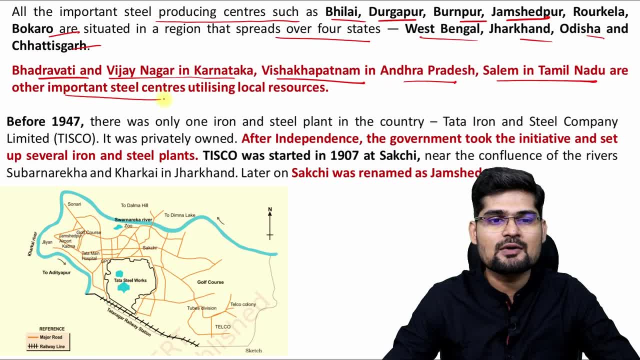 vishakhapadnam in andhra pradesh, salem in tamil nadu are other important steel centers utilizing local resources. the most famous one, if you observe, before 1947 was tisco tata iron and steel company, and after independence the government took to the initiative to set other iron and steel plants. 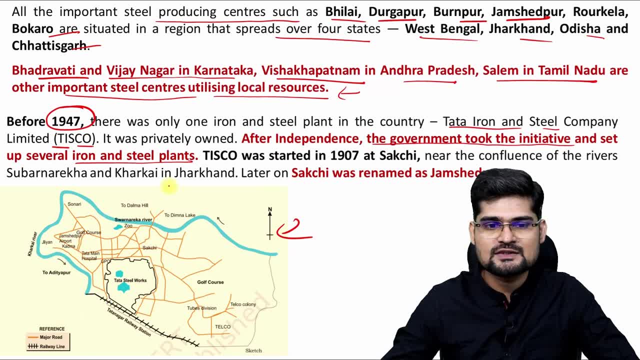 now this is the sketch map of tisco. if you have ever been to the place called jamshedpur, you'll understand this here. so earlier it was called sakshi, which was renamed as jamshedpur right in 1907. tisco was started here and this is the plan map. here you have steel works and you have this. 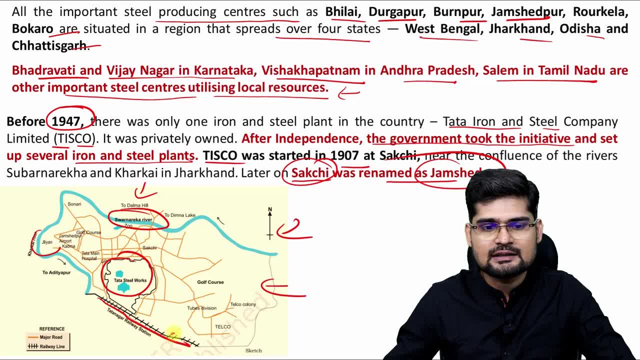 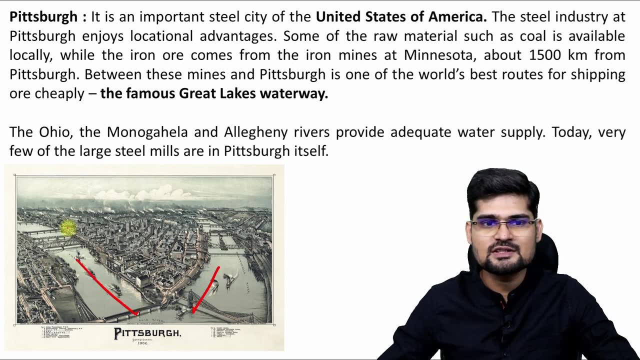 suvarna, rekha river, kharkai river and the area connected with- observe here- is transportation, the railway line, right, so that's how it was made in that particular location. now, similar kind of locational advantage, if you see, is pittsburgh. these two rivers, if you observe here, pittsburgh enjoys the locational advantages in us. 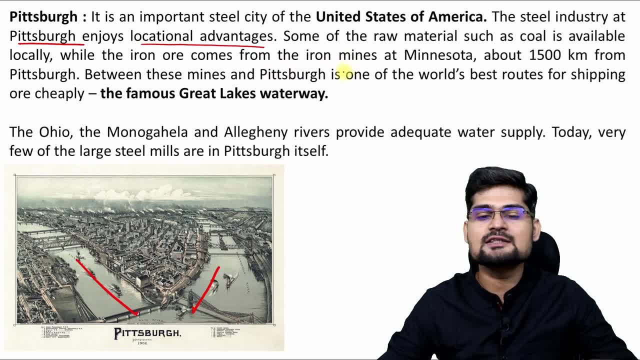 right and it takes iron ore as long as 1500 kilometers right from minnesota iron mines. they get these raw products and then it is processed at pittsburgh, right so famous great lakes waterway. this is what gives its locational advantage, right so everywhere in the world where 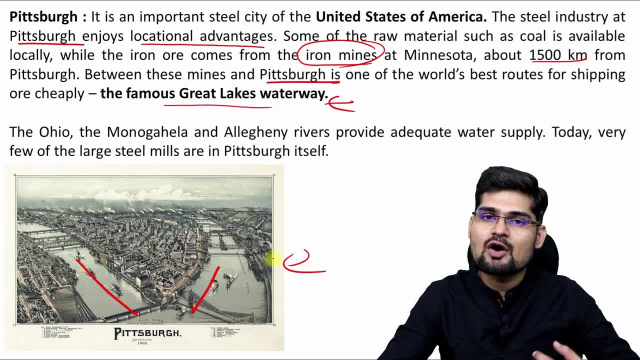 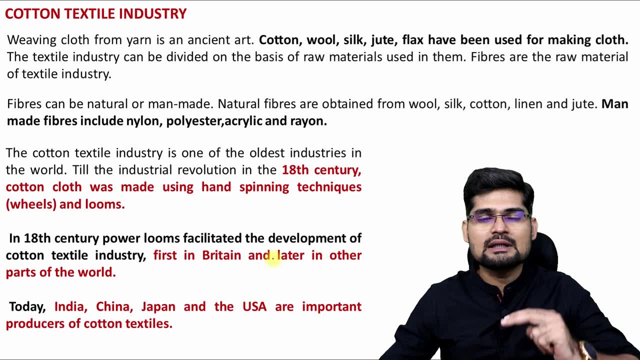 iron and steel industry is located, location, raw materials and its transportation and circulation becomes really, really important right now. come to next kind of industry, which is cotton textile industry case study. so here, if you observe, weaving cloth from yarn is an ancient art right. cotton, wool, silk, jute, flax- these have been used since ancient. 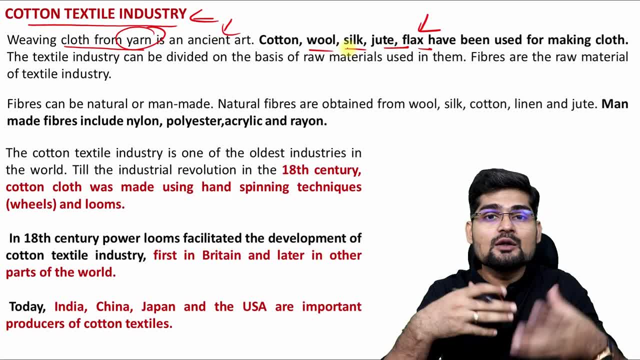 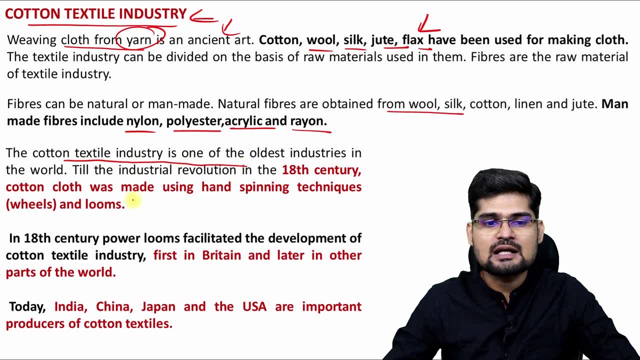 times to make make cloth. so what happened during colonialism? it was now mechanized and industrialized. so what happened earlier? the cotton textile industry, which was running on a hand milling, made looms, were now converted to power looms first time in britain. so it was now running on power it. 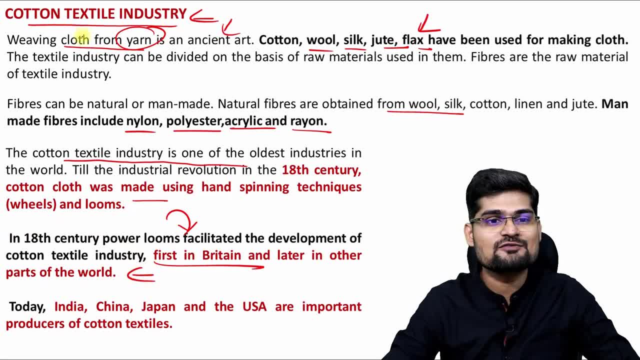 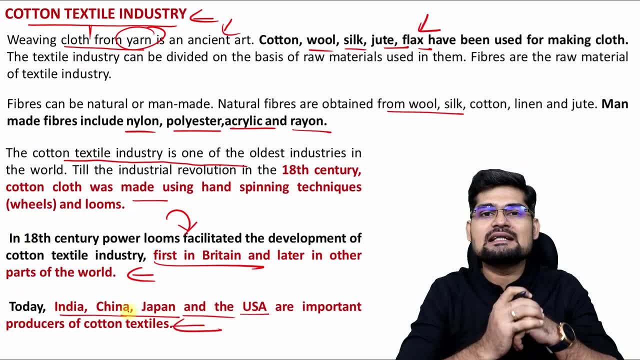 was more mechanized. so there comes the industrial revolution from cotton textile industry in 18th century, right? so india, china, japan and usa importantly produce the cotton textiles at the most in the world, right? so if you observe this list here, it gives us the countries, their ranks. 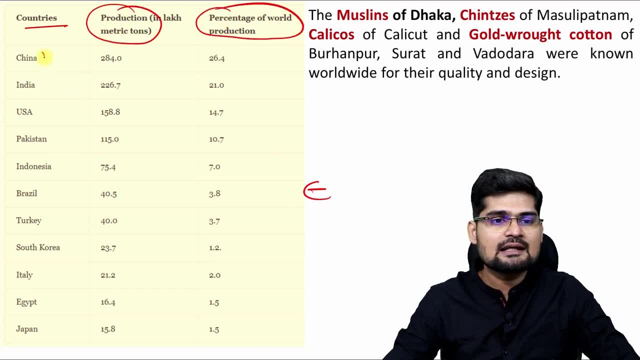 in terms of production and also percentage of the world, china ranks the top. then is india, then us, pakistan, indonesia, brazil, turkey, south korea, italy, egypt, japan. so if you observe here this, these are the major countries which are producing the cotton textiles. muslims of dhakka, chinsis of 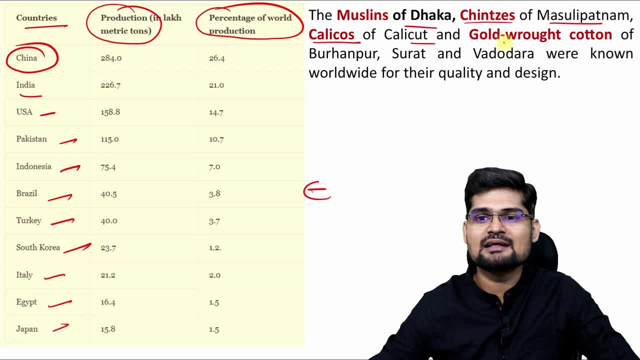 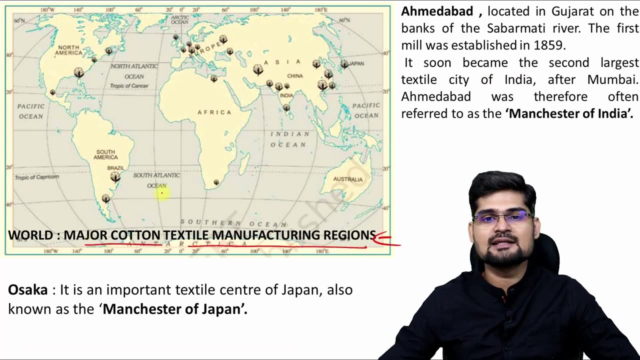 masuli patnam. then you have calicos of calicut. gold rot cotton of burhanpur, surat and vadodara were known worldwide for their quality and design. these are the famous indian ones. remember that right. so now, if you observe world major cotton textile manufacturing regions, 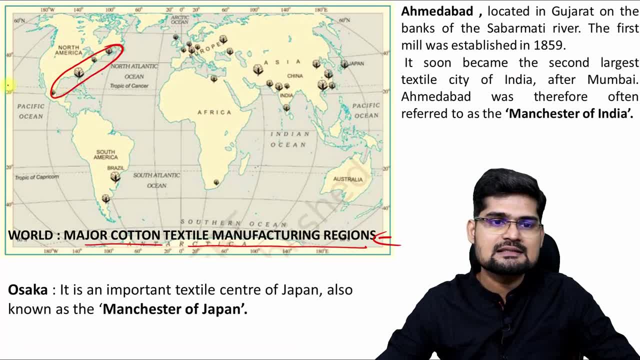 on them map. there is a pattern. these are the areas in us. then you have this western europe here industrial revolution, then some portions in central asia, hugely in india and china, if you observe here some portions in south america as well and south africa as well. so this is majorly into this. 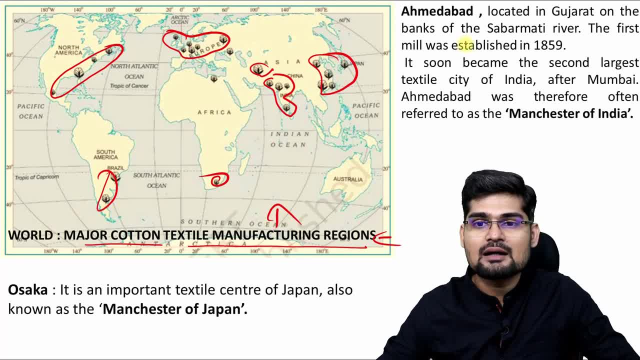 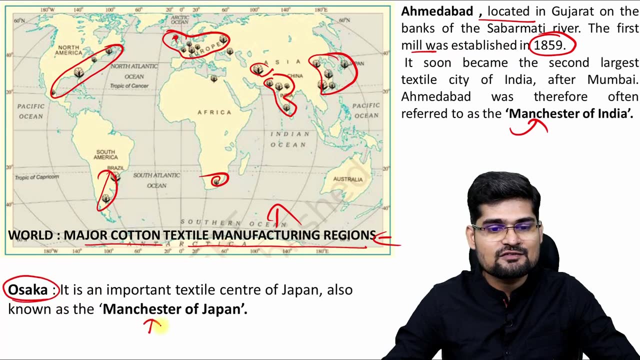 manufacturing of cotton textile, and amitabad in india, in the state of gujarat remember, where in 1859 the first mill was established, is also known as manchester of india, because manchester in uk is very famous for producing the cotton textile right then. in japan, osaka is very famous, it's called 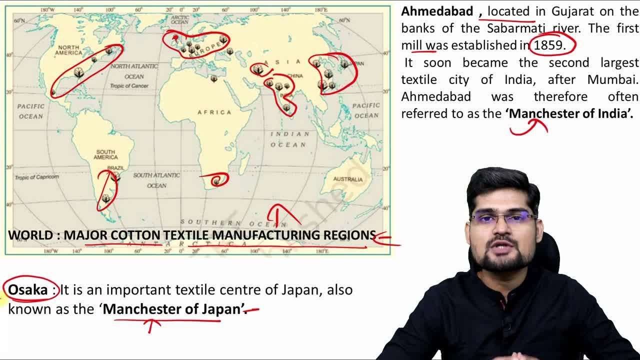 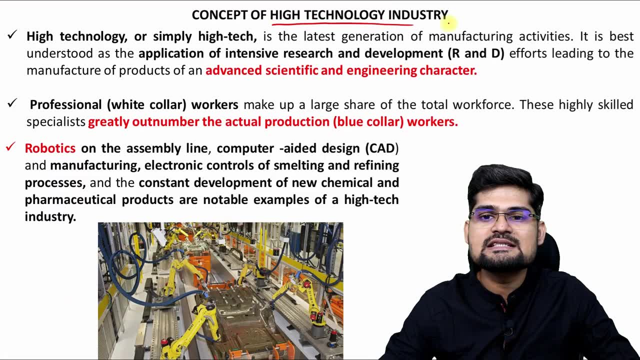 manchester of japan, right, so these are the places which are the major cotton textile producers of the world. and then comes the concept of high technology industry in secondary activity, in economy. so high technology, or simply high tech industry, that we say: what are these? these are based on intensive resources. 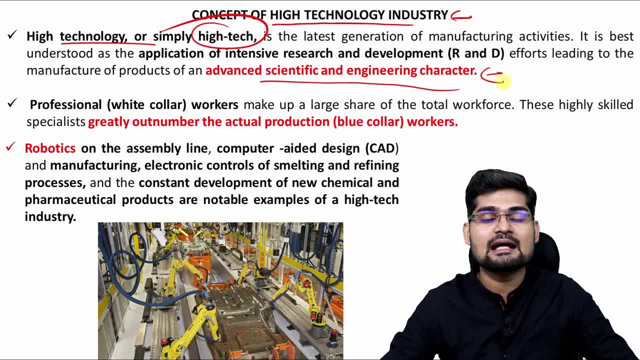 research and development and advanced scientific and engineering characteristic, for example, professional white collar jobs. white collar workers make up large share of the total workforce right, the engineering graduates, the young minds, the tech scientists right, and they are highly skilled specialists. so they greatly outnumber the actual production that is blue collar workers right. so 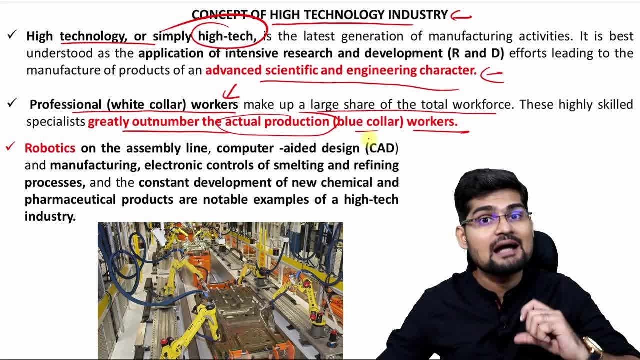 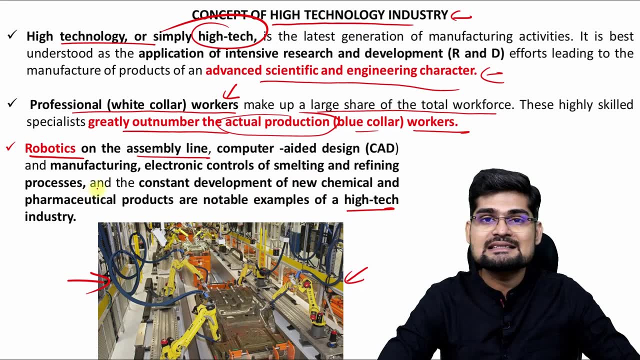 here that typical labor job is not required. here skilled labor job of high end is required. so robotics are one of the things that are done in assembly line. if you observe this diagram here, this is a high tech industry which is producing cars, which is producing machines. so this has overtaken the world in modern science and technology development. 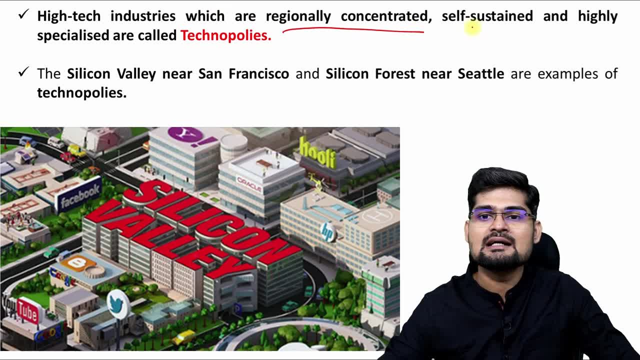 alongside so high tech industries which are regionally concentrated, self sustained and highly specialized, are called techno police. now, remember this word called techno police. techno police are what these are: the hub or the agglomeration of such industries, which are all high tech. so, for example, silicon valley near san francisco, the very famous 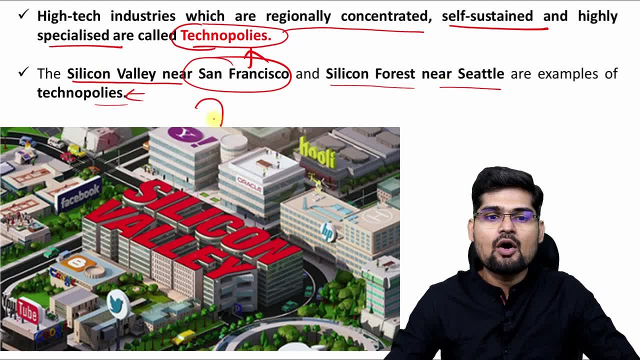 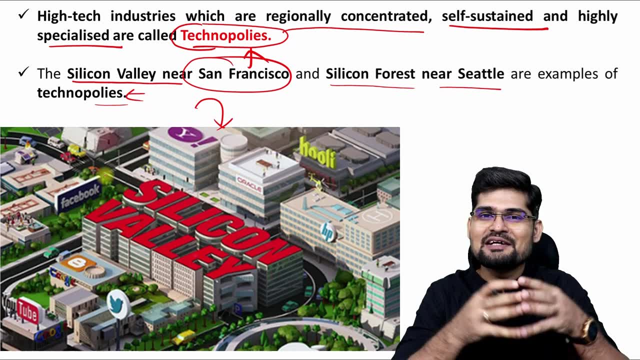 silicon forest near seattle are examples of techno police. all the high and techno crafts and all the meetings and all the world phenomena is taken over by silicon valley. right from the microsoft to google to the name it, all the high tech industries are having their headquarters or having 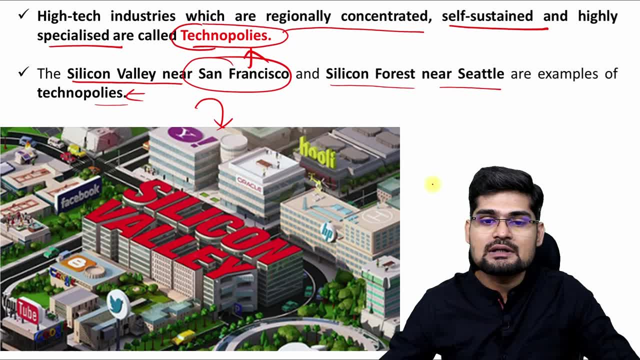 their offices in silicon valley, right, so it becomes really important in today's world at high tech industries are established, if you observe, from youtube itself to others like hp and several oracle, yahoo, face- all of them are there in silicon valley, if you observe, right. so these are what these are not. 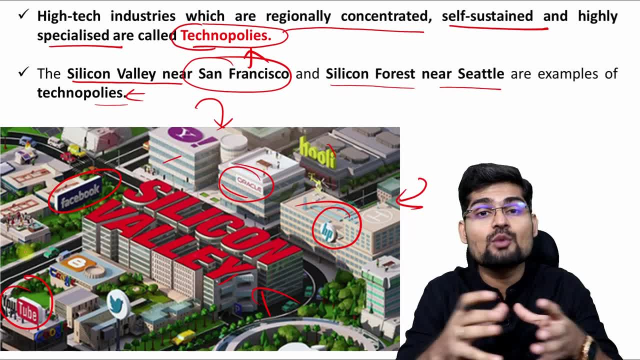 based on the labor jobs. like other industries, these are skilled, white collar labor jobs. softwares, technology, robotics, engineering- that's what it is driven through, right. so that's what we say is high-tech industry and it also falls under the secondary activities in the economy. so most 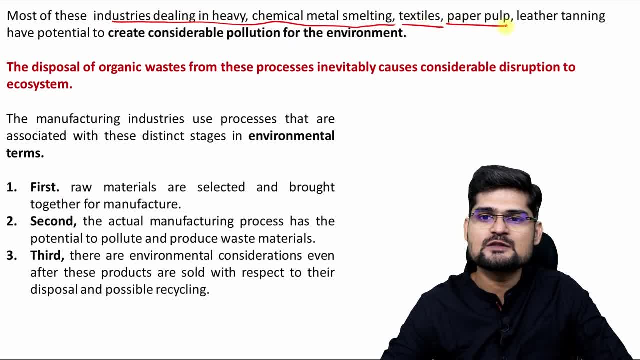 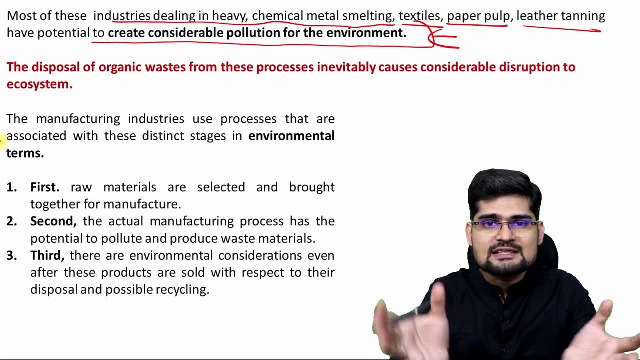 of these industries are dealing in heavy chemical metals, melting, textiles, paper pulp, leather tanning and create considerable pollution to the environment. as we know, it is talking about the all kinds of secondary activities, not just the high-tech right. so high-tech industries are the least polluting, if you observe, out of all the secondary activities, but rest of them definitely. 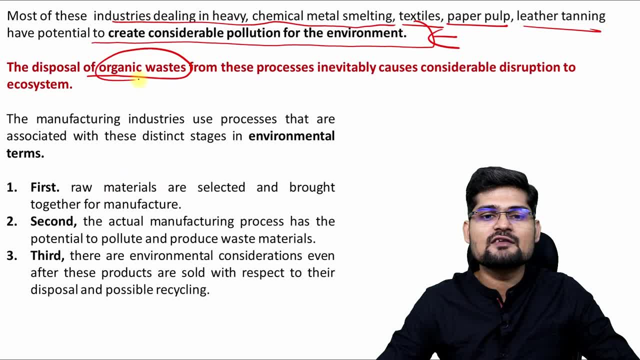 have a footprint right. so disposal of organic waste from these processes are of great concern right now and manufacturing industries use process that are associated with these distinct stages in environmental terms. first is raw materials are selected together to manufacturing hub and then actual manufacturing process. has this potential to? 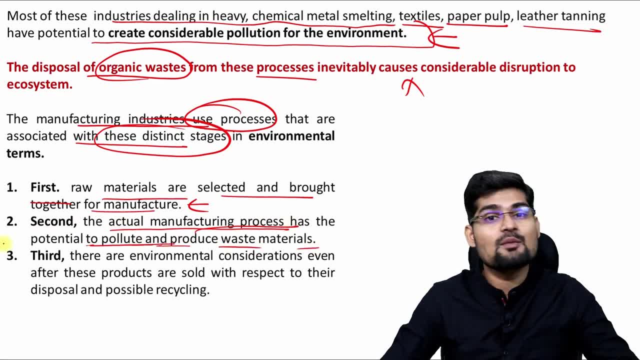 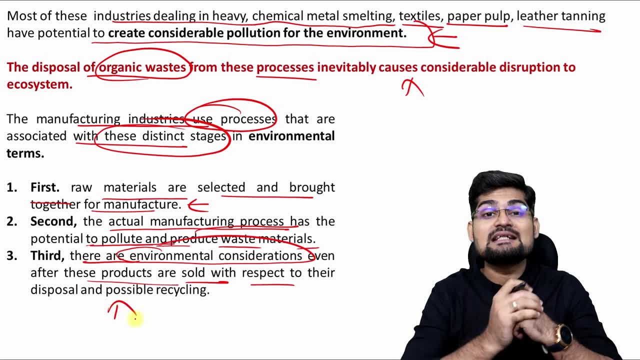 pollute and produce the waste material. that's where it is produced, not at the raw material end. and then, third, there is environmental consideration even after these products are sold, with respect to their disposal and possibly recycling. that's why we say, in sustainable development, that is reduce. 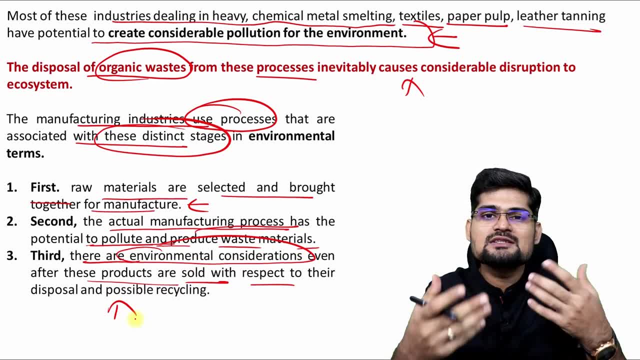 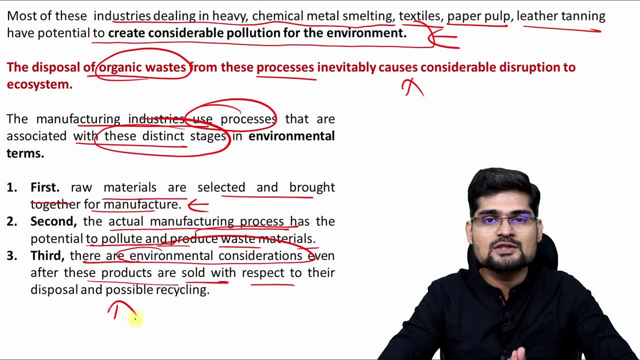 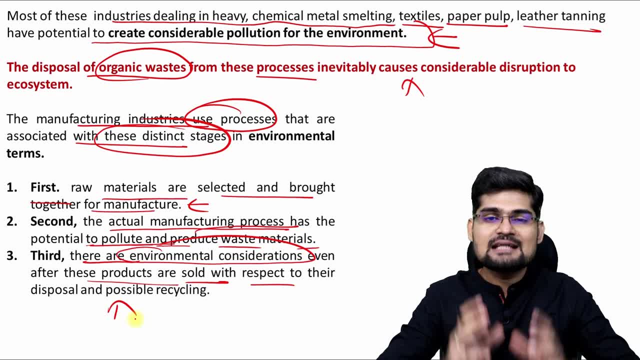 producing more footprints on the planet. right? so that's how the concept is linked with our carbon footprint analysis as well. so the idea is that secondary sector is the major sector of economy that is also, at the same time, affecting the environment. that's what is to learn from here. 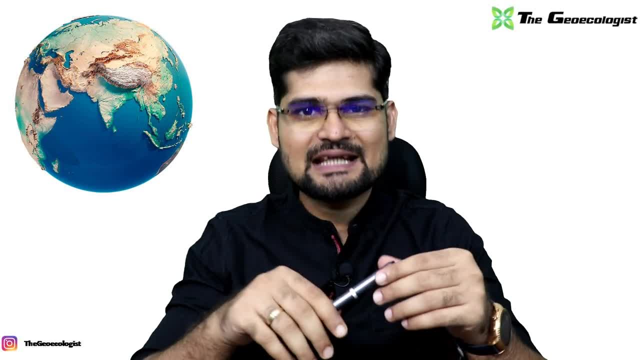 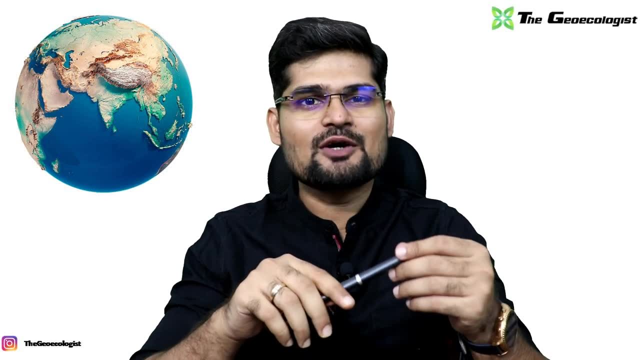 so now when we have learnt about all the concepts related to secondary activities in the economy, various case studies, examples: in the sessions to come we'll be talking more on different topics of geography. so stay tuned, stay safe, keep watching and learning, and don't forget to share the videos. with others as well.